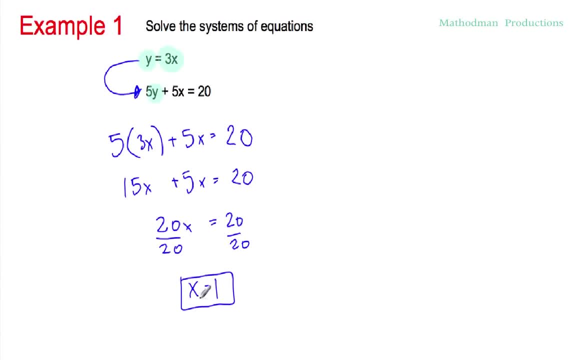 That's half the problem done right there. Now that we have a value for x, it doesn't matter which equation you choose, Just substitute that value in so you can solve for y. It's usually best to choose the simpler equation. I'm just going to rewrite it right here: y equals 3x. Now instead. 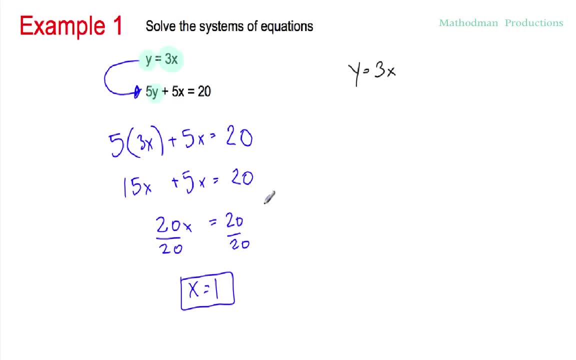 of x. we have a value for it. We have it as 1.. y equals 3.. Substitute it again, 1., And simplify: y equals 3. And our problem is solved. Here's my solution: x equals 1. And y. 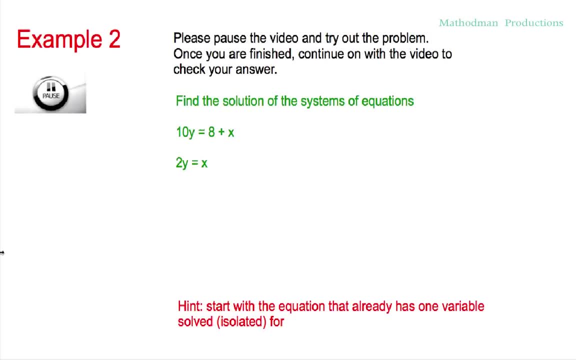 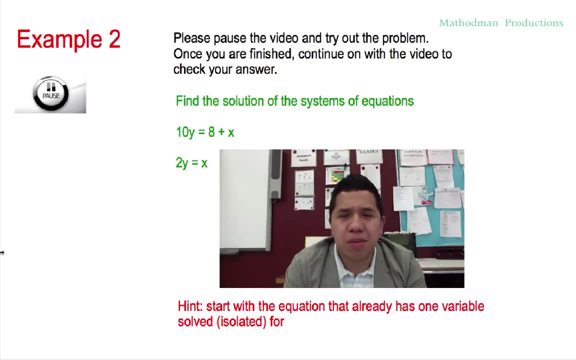 equals 3.. Please pause the video and try out the example And hit play once you're done, And an explanation and your answer will be given to you. So don't cheat, I'm watching you. Anyways, before I let you try the problem a little hint below, Start with the equation that: 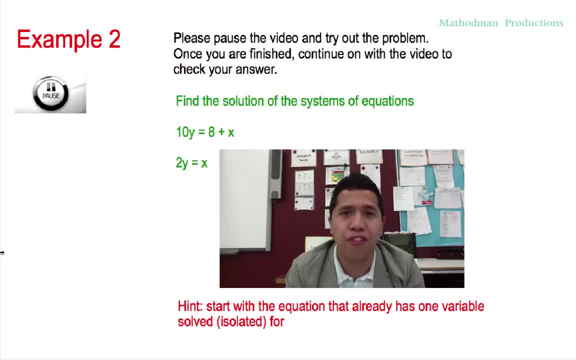 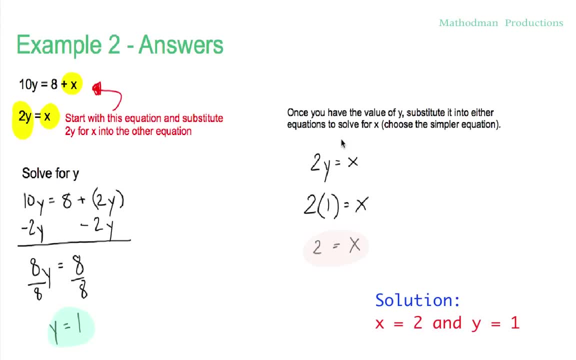 already has one variable solved for, Or one variable that's isolated already. I think you can tell. So hit pause right now. Here is the answer, for example: 2. First, start off with the easier equation, That's the one on the bottom: 2y equals x And substitute it in to the other one. 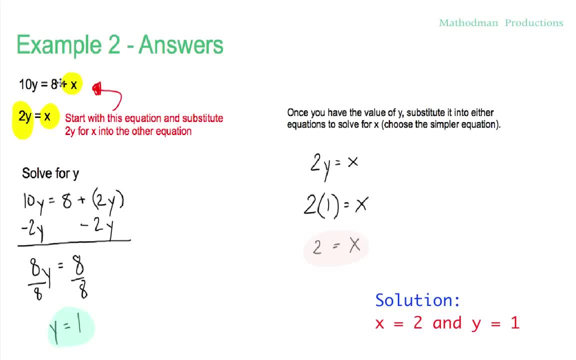 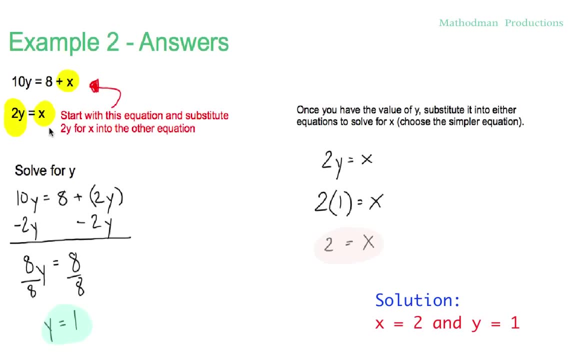 Substitute 2y for wherever you see an x in that top equation. That's what I did right here- And just solve for y Pretty easy. Once you have the value of y, substitute it into the other equation. It doesn't matter which one Solve for x. Choose a simpler equation, It'll make your head hurt a. 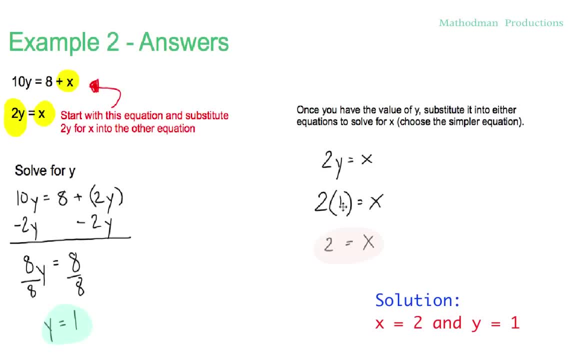 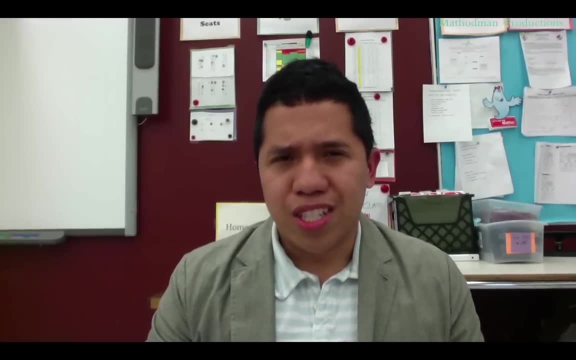 little less, So 2 instead of y. We're going to plug in a 1 equals x And simplify from here: And x equals 2.. That wasn't so hard, was it? But anyways, if you're still confused, I have another.